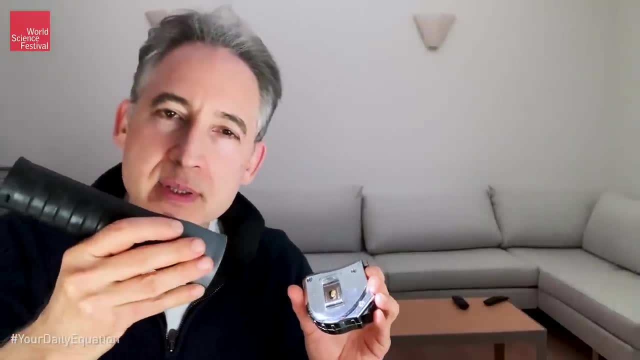 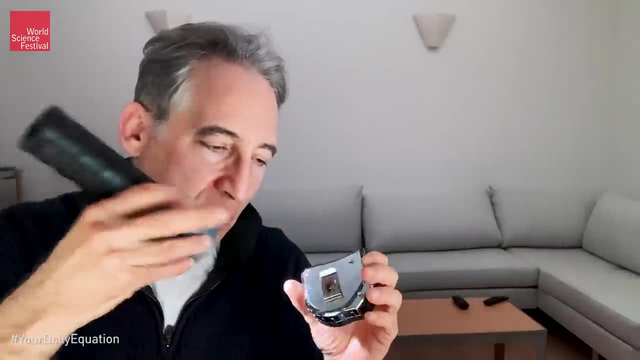 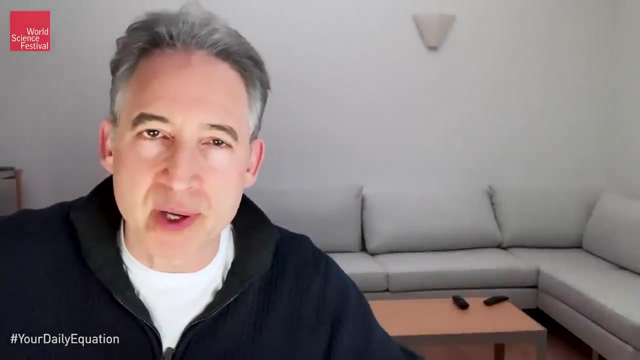 the surface. And the idea is that if I do this in the right way, in the right experimental setup, then the light from the source can cause electrons from the surface to be ejected Outward. So this in itself is not a particular puzzle, because after all, light is an electromagnetic. 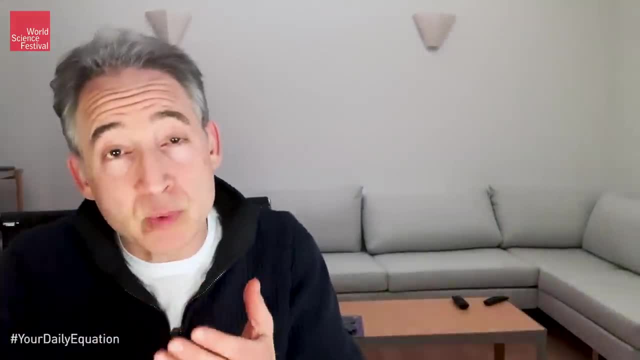 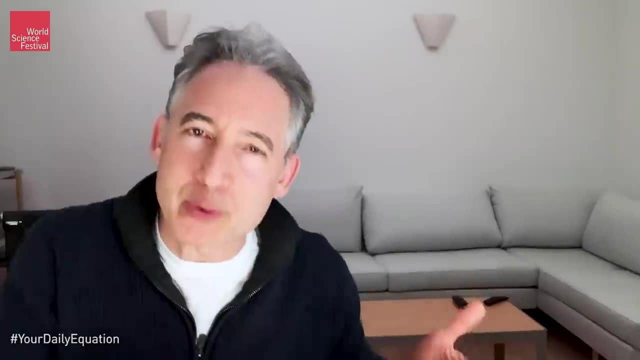 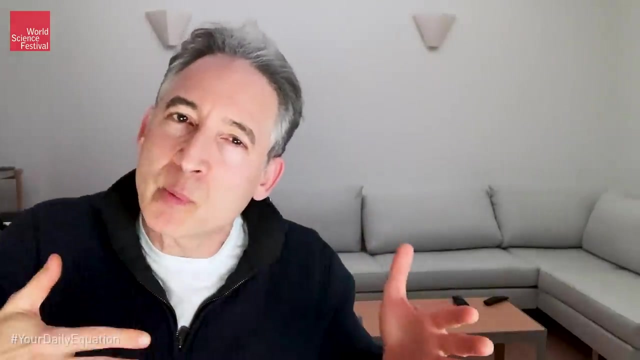 wave, An idea that we will also discuss subsequent to the discussion today, One of our other discussions of Maxwell's equations. But light carries energy, and so energy slams into the metallic surface. The electrons are loosely bound to that surface, and the energy from 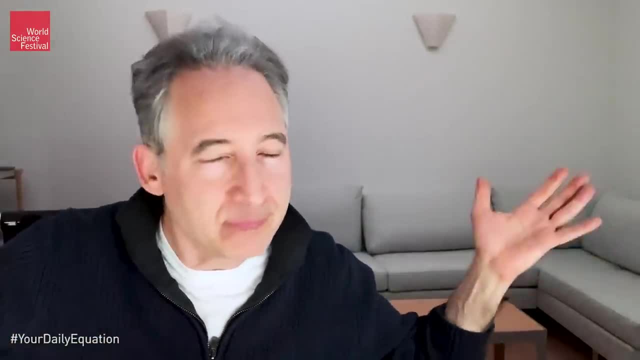 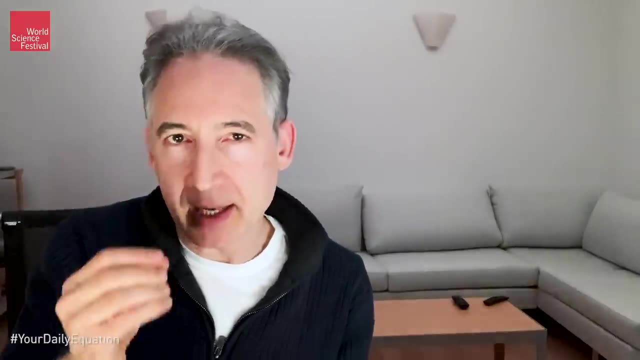 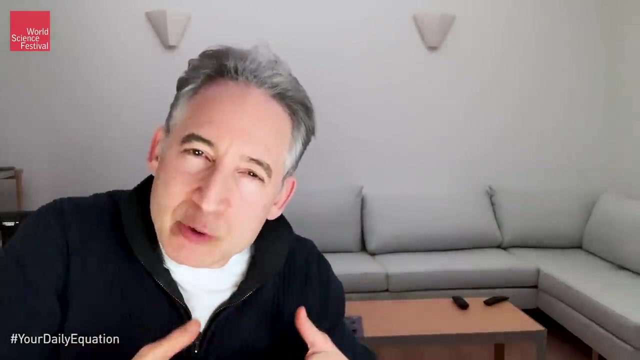 the wave can knock the electrons free. Not particularly puzzling at all. But what is puzzling is when you look at the details of the data, Because you would think, or at least most people would think, that the kinetic energy, the energy that the electrons have their speed when they leave the surface, should 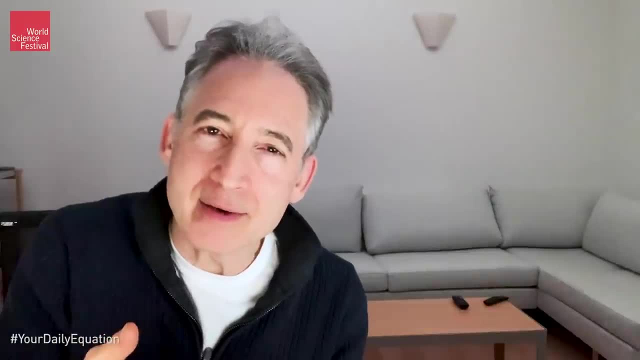 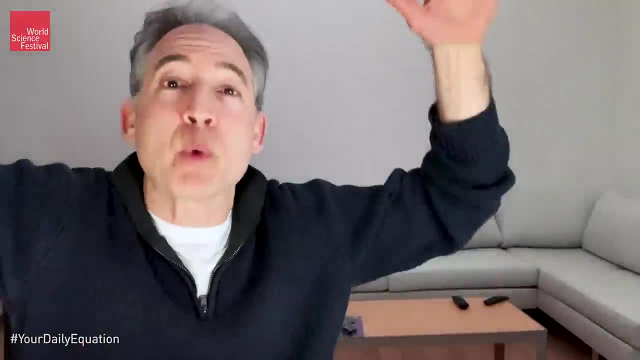 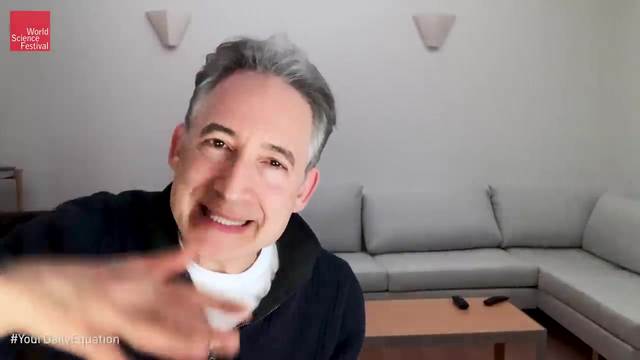 be determined by the intensity of the light. Right, After all, light is this wave. and the intensity of a wave. the intensity of an ocean wave is given by the intensity of the energy of the light, Given by its amplitude, the ups and downs of the wave. Similarly, the ups and downs 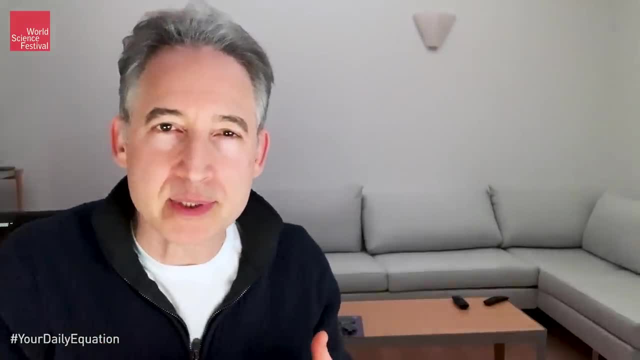 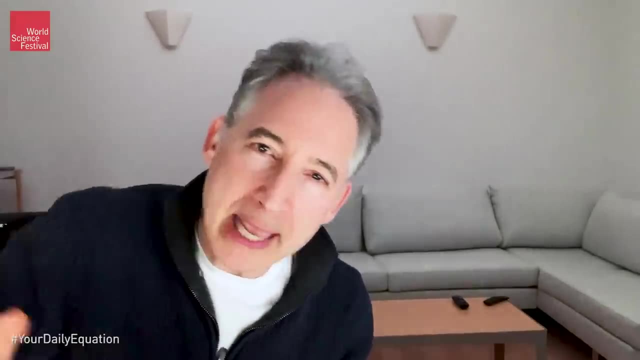 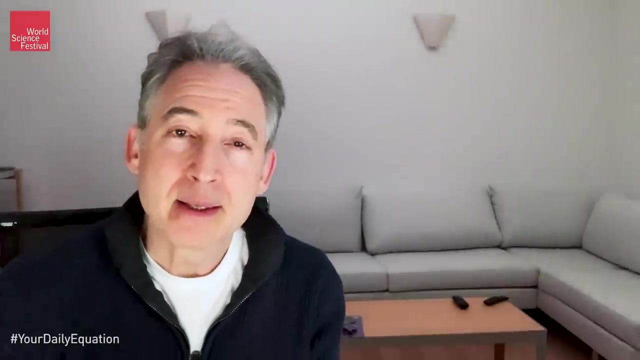 of the electric and magnetic fields that comprise the electromagnetic wave that is light, the ups and downs, the amplitude that should determine the energy of the light and that should determine the energy of the electrons that are ejected. But when you look at the data, that's not at all the case. You know what determines. 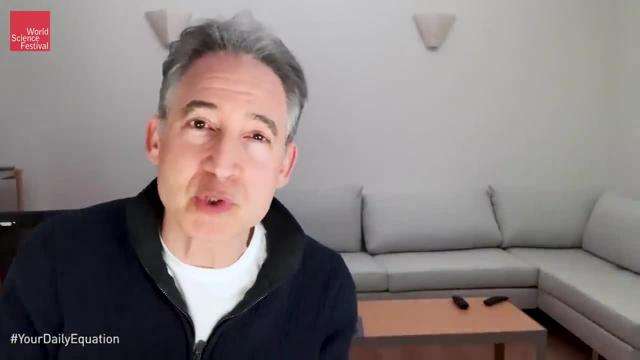 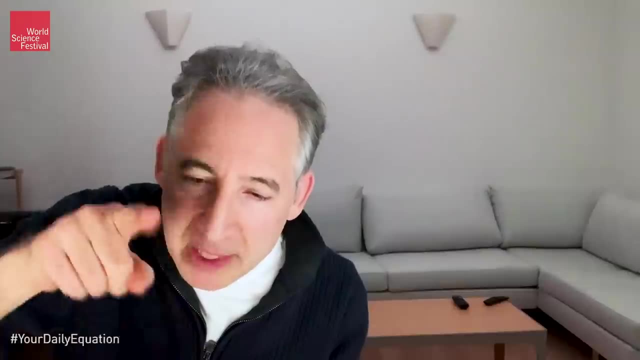 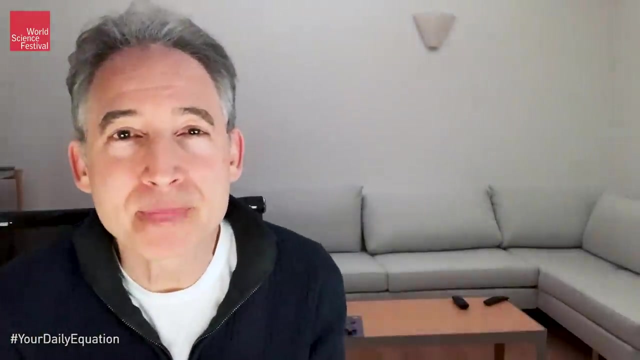 the kinetic energy, The energy of the electrons that are knocked free from the surface. The color of the light, Its frequency, that is, how quickly it oscillates up and down, determines at least the maximum kinetic energy of the ejected electrons. The intensity of the light does determine. 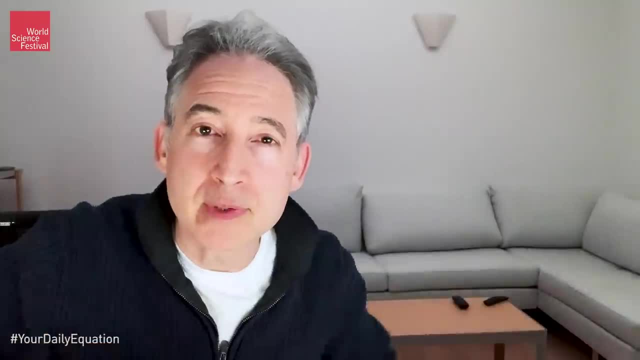 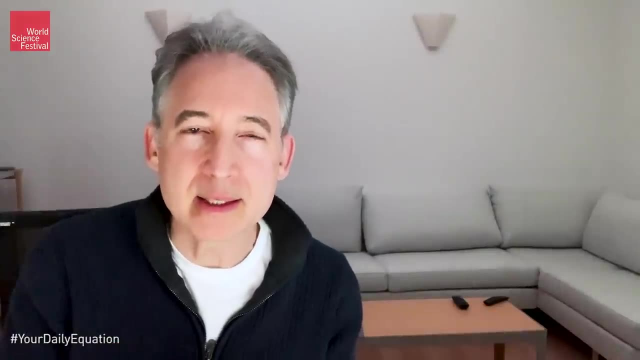 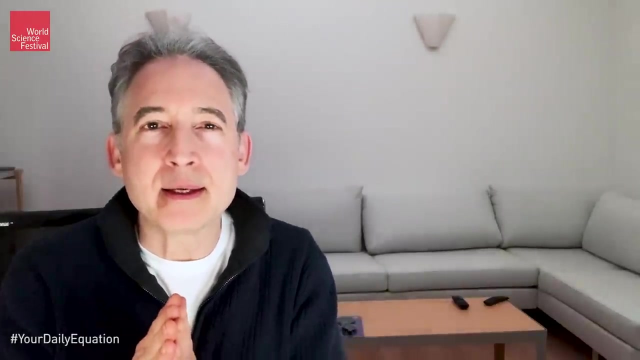 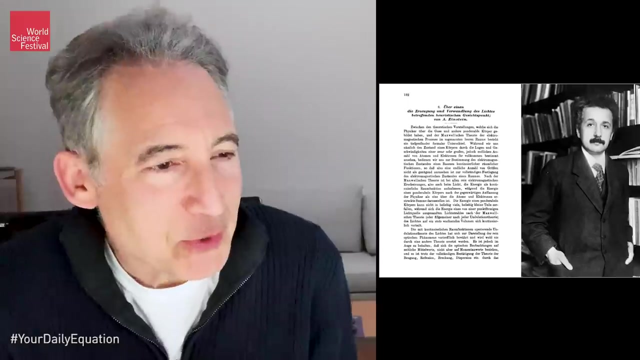 something else. It determines the number of electrons that are ejected from the surface, But their energy comes from the color of the light. So this was a puzzle that Albert Einstein starts to think about, And he ultimately comes up with a solution, And that solution I can actually show you the paper right here. So 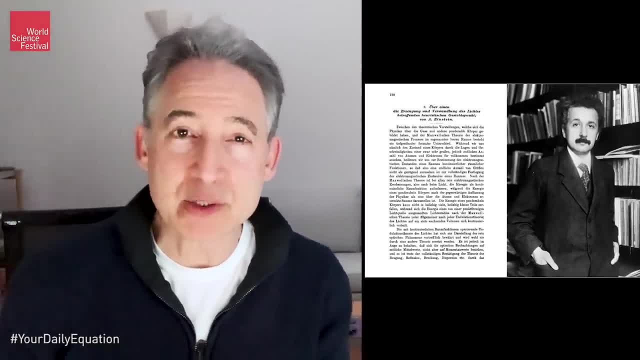 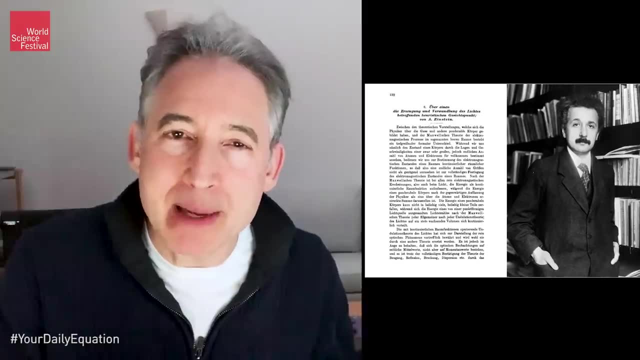 this is his 1905 paper on the photo electric effect. 1905 is often described as Einstein's miracle year. He writes a handful of papers. Any two of them he pays his kinds with 100% percent. So this is in 1905. He forges his own paper in 1905. And he And then he Lawson writes his^^. The послеnvers repent. I'll give you the answer in 30 secondsl. I'll read you the reply of the next. nicely thời, eure Motorola vigilante in the space. I'm even nervous. I'm coming to you, Thomas. 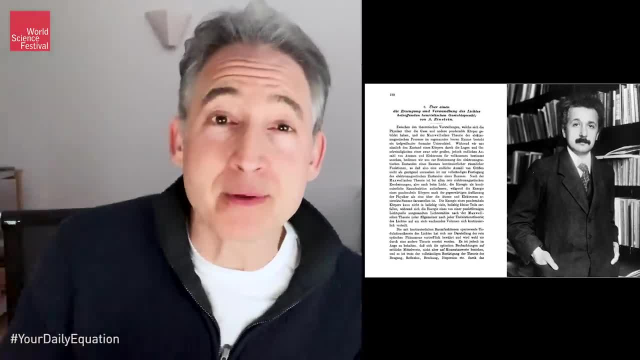 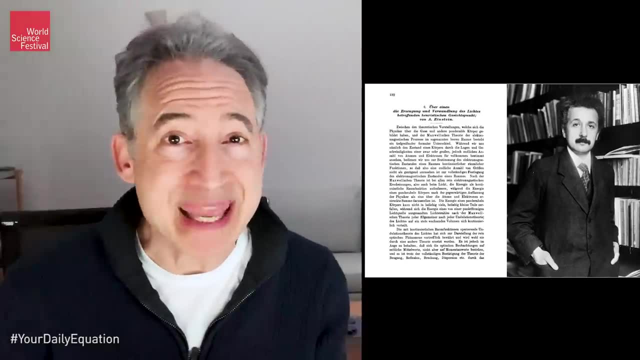 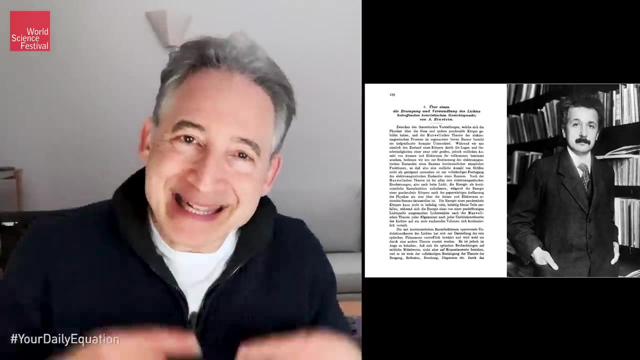 any two or three of which could have themselves received the Nobel Prize. but it's actually this paper, not his paper on special relativity, not his paper on equals mc squared. it's this paper for which he receives the 1921 Nobel Prize in physics, and it is in this paper that he unravels. 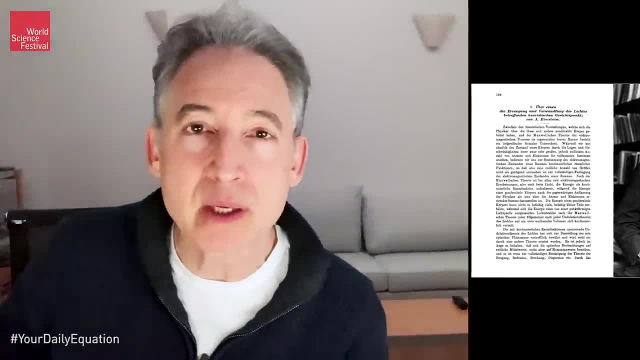 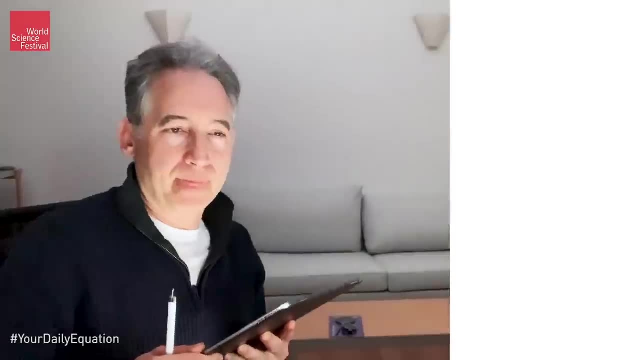 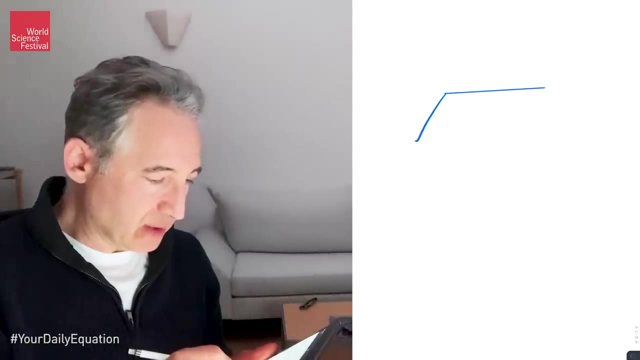 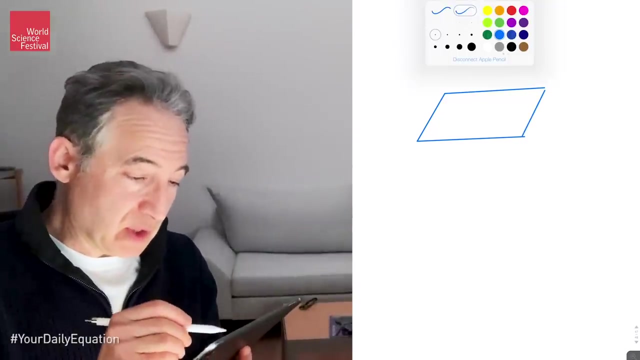 this paradox of the photoelectric effect and let me just describe to you what he finds. so the picture- let me just bring up my iPad here. good, so the picture that we have, at least that we're trying to figure out here. imagine that this is my metallic surface and let me just describe light as a wave coming in. so this is the 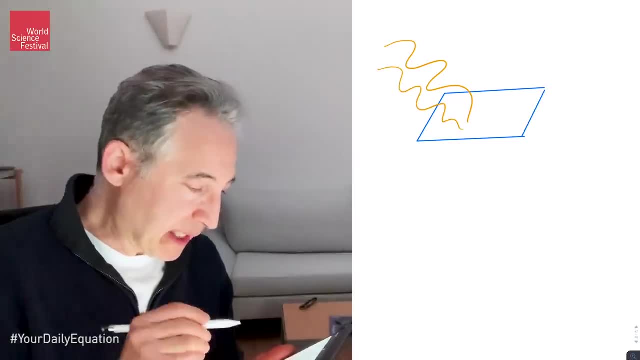 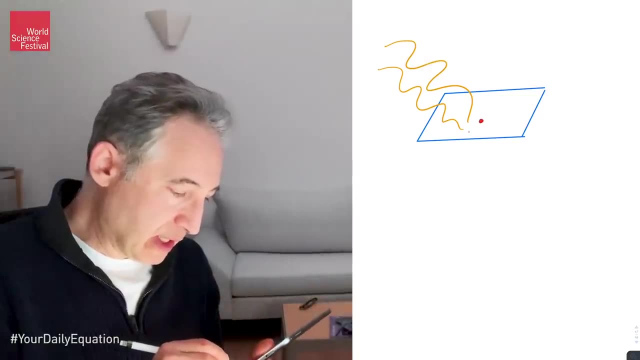 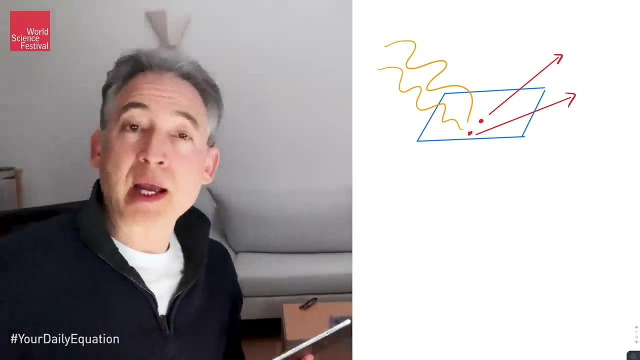 usual picture. you've got this electromagnetic wave slamming into the surface and you've got a water drop and a real light and a real wave, and a real wave and a real low air pumping out of here, say, let's say, little electrons in here and these electrons are flying out and, surprisingly, 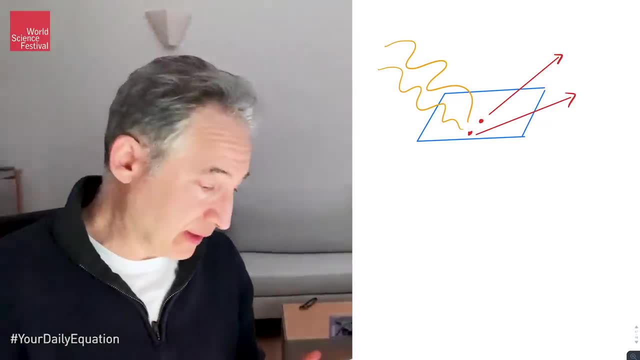 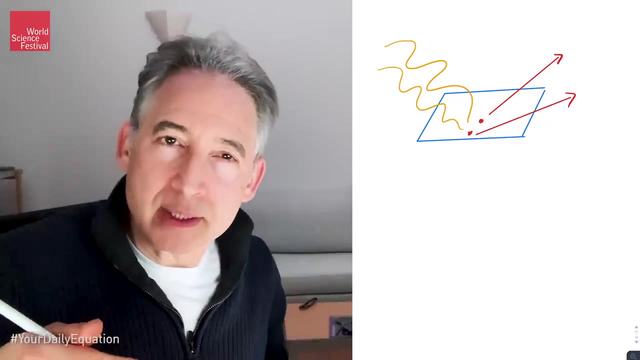 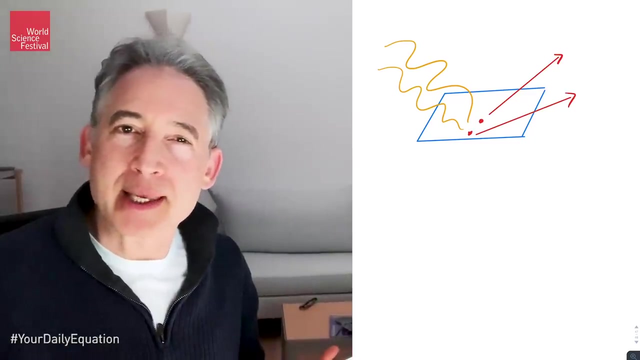 their energy is determined by the color of the light. How does Einstein explain this? Well, Einstein makes use of a different image of light, a different picture, a different description of what a beam of light actually is. He actually goes back to an idea that we can trace to Isaac Newton himself, where Newton 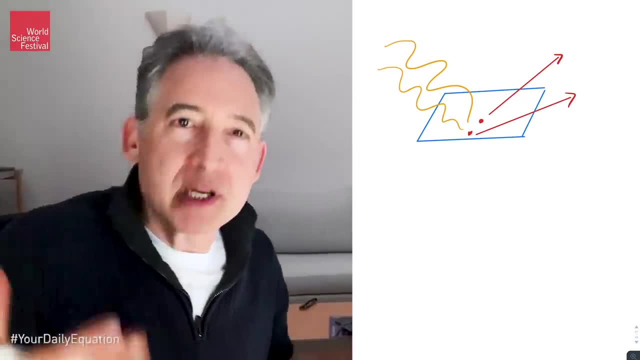 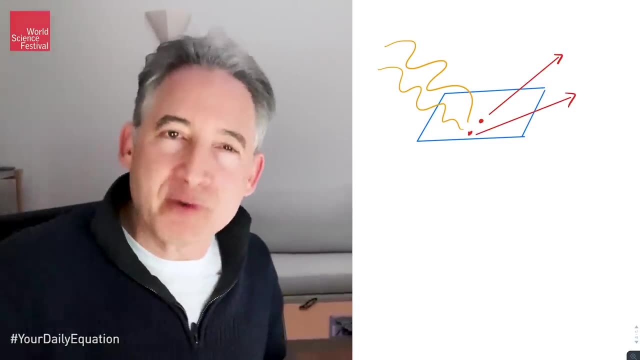 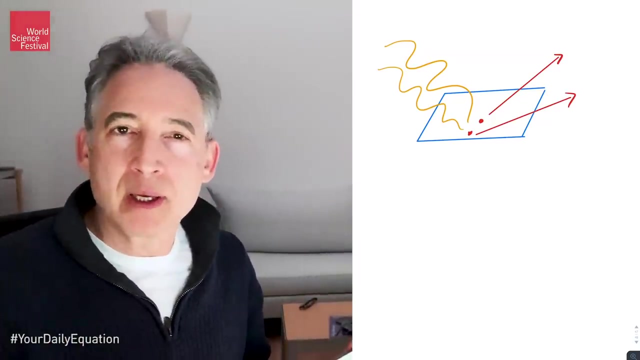 thought that light was actually made of a torrent of particles. We call those particles of light now photons, so let me use that language- A torrent of photons as opposed to some kind of wave-like phenomenon. But that idea was dropped when people like Thomas and Maxwell showed, apparently, that 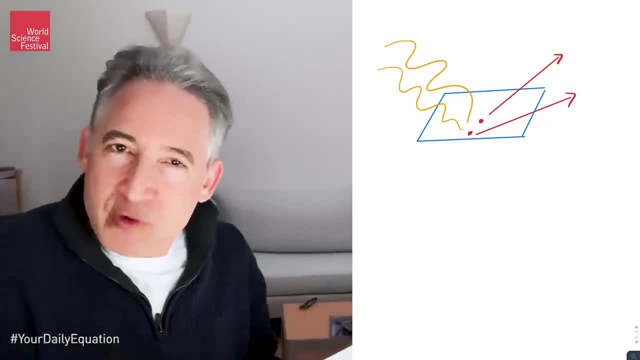 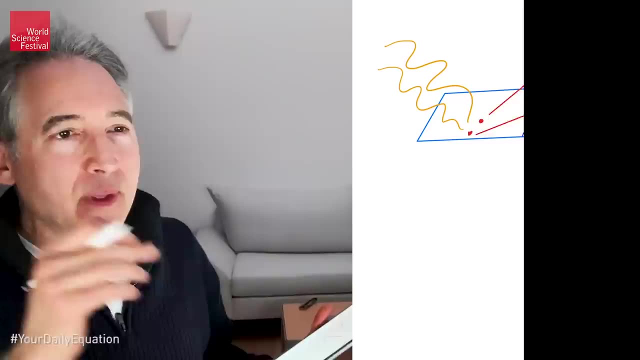 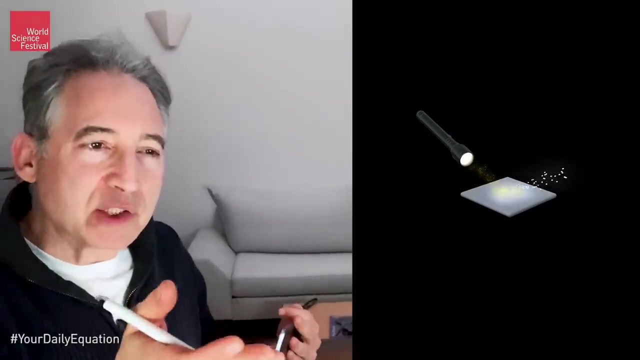 light is light. Light is an electromagnetic wave, but Einstein kind of goes back to that old idea of light as a stream of particles. In fact I can show you in this sort of fancier version of the demonstration now done in animation: You see that from the flashlight, that beam of light, Einstein says it's actually a stream. 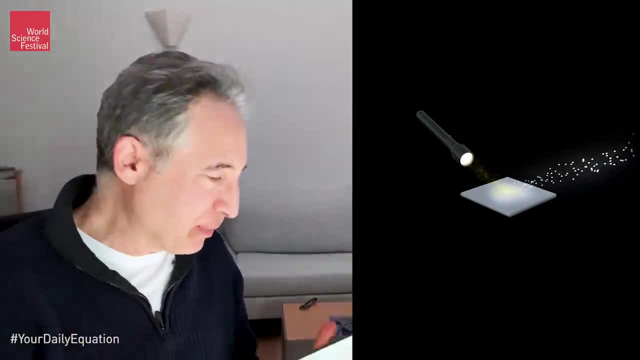 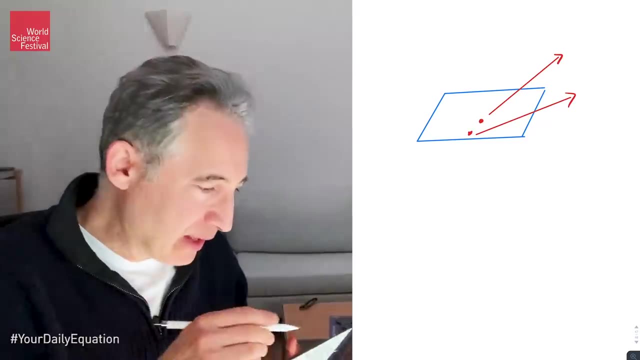 of particles. Now, how does this resolve the problem? Well, let me go back to this picture over here. Let me erase this idea. Let me erase this idea of light as a wave and, in its place, let me describe it as a. 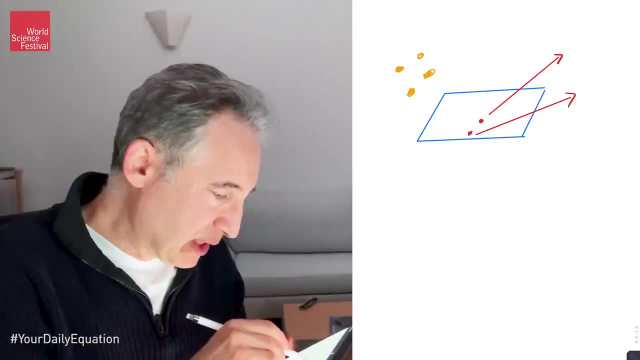 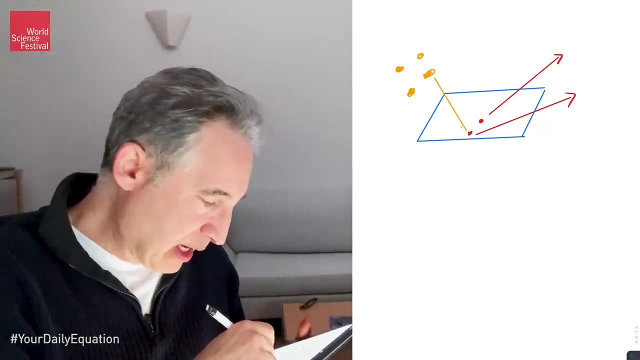 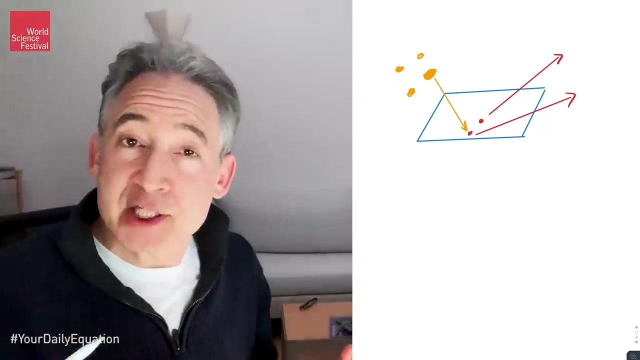 collection of particles, each of which is flying down to the surface. Let me focus on one of them- this guy over here- and imagine what's going on when a photon hits the surface and ejects an electron. is a collision between the photon and the electron. 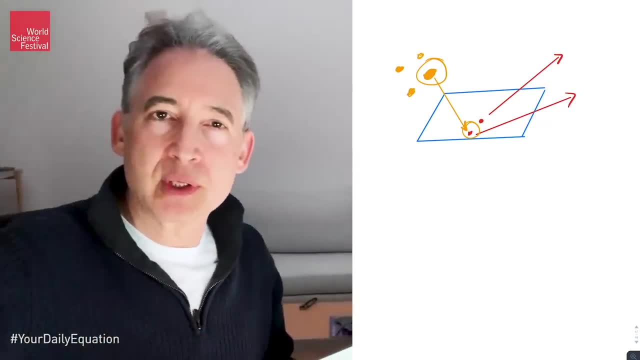 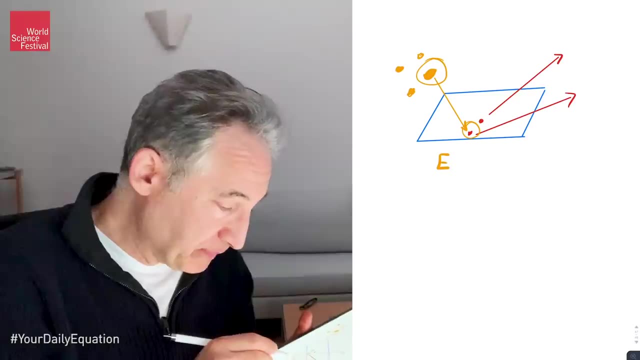 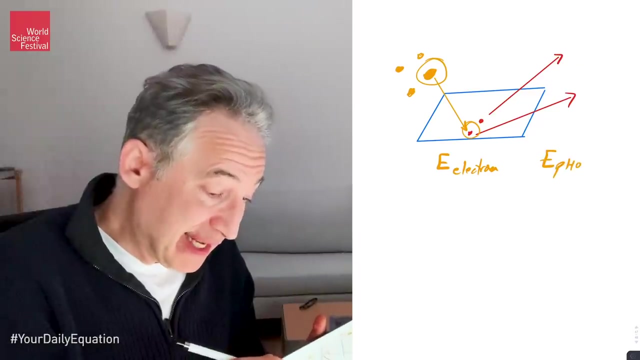 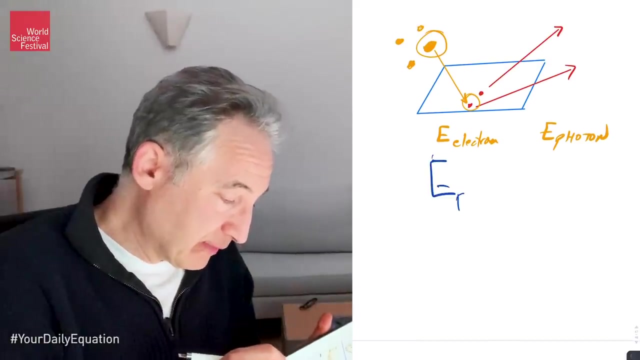 and that's one-to-one collision. A collision is what ejects the electron and clearly then the energy of the ejected electron, the energy of the electron will be determined by the energy of the photon that hits it. Now Einstein says, in order to match the data, that the energy of that photon must. 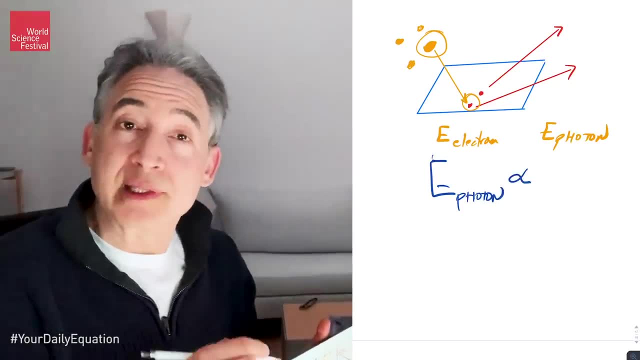 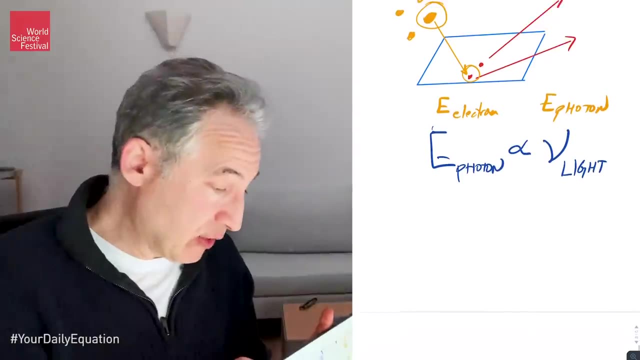 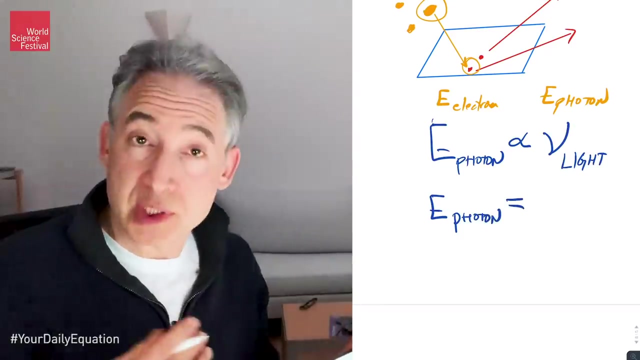 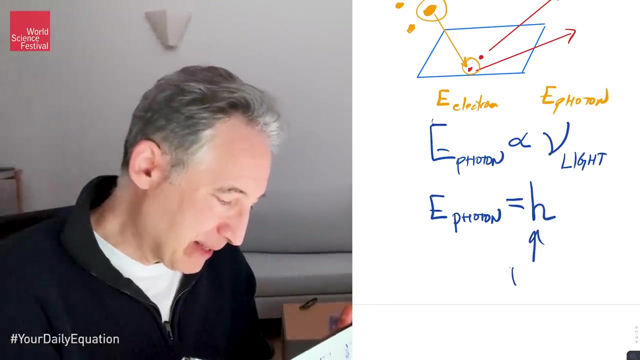 be proportional to the color of the light, Which is the frequency of its oscillations. And indeed you can go further and make that proportionality into an equality, which is today's daily equation, by using a number called h, which is known as Planck's constant. 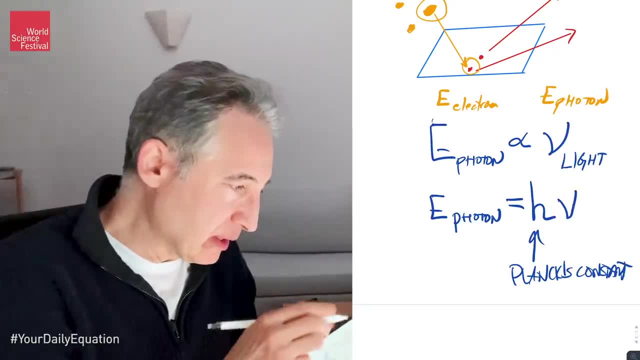 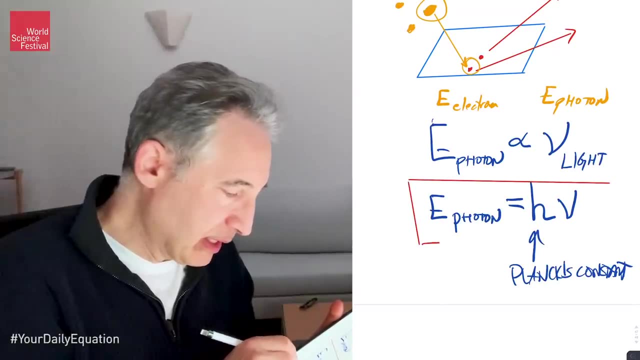 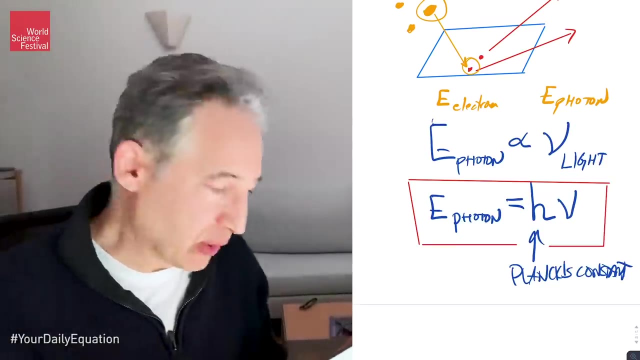 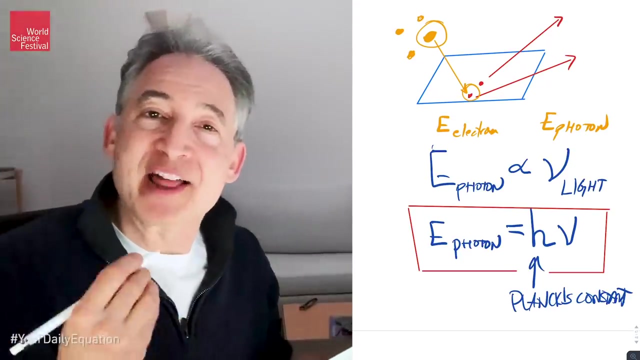 after Max Planck And the equation therefore. The equation therefore that he comes to is: E equals h nu. And this idea of light as a collection of particles explains why it would be that the kinetic energy of the ejected electron would depend on the color of the light. because 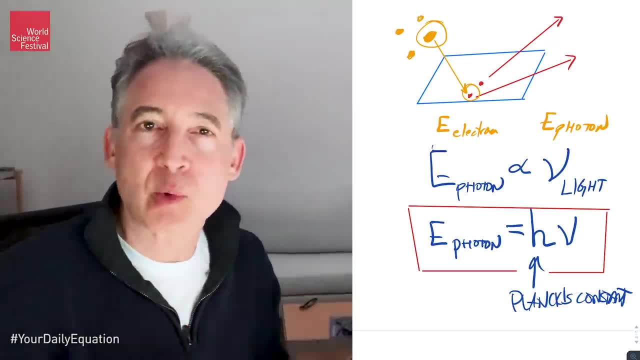 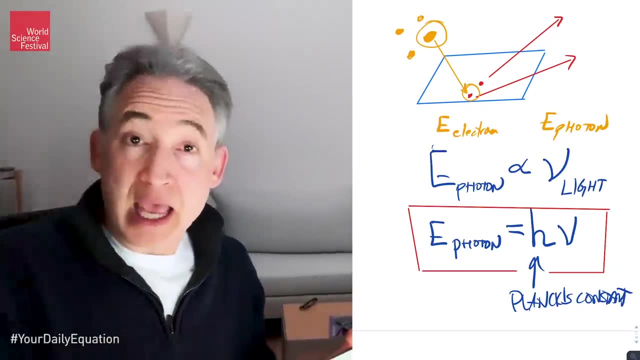 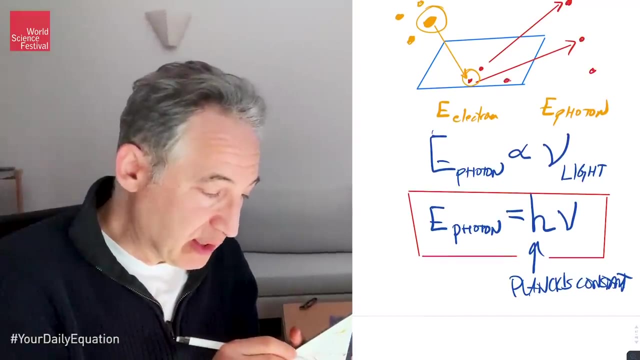 the energy of each individual photon via this equation is dependent upon the frequency of the light, dependent, therefore, on the color of the light. And we can go even further. Why would it be that the number of these electrons that are ejected is dependent upon the intensity? 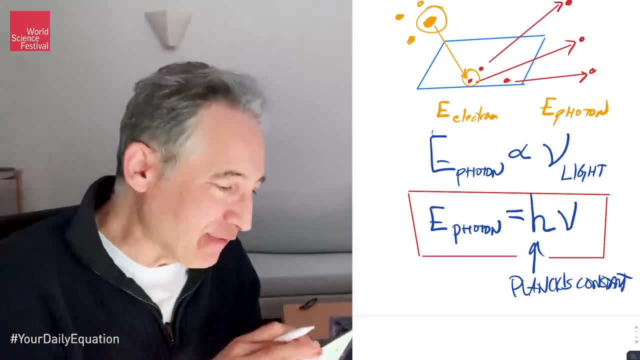 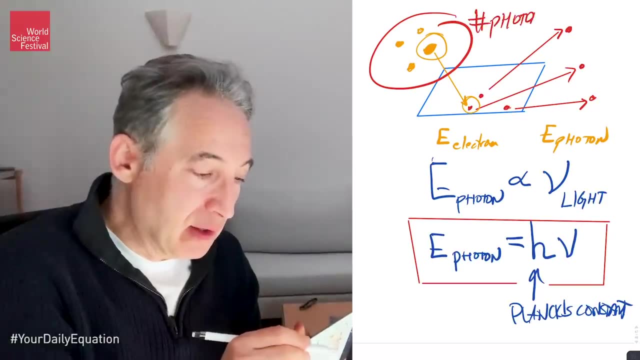 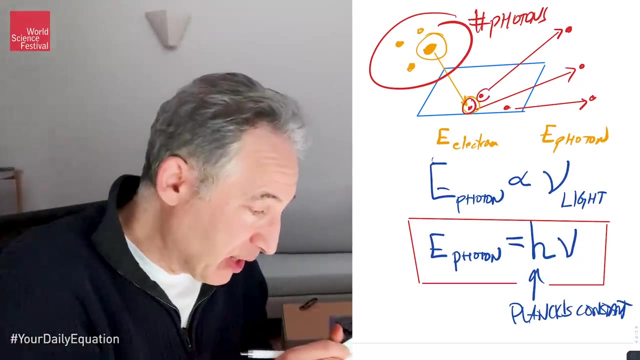 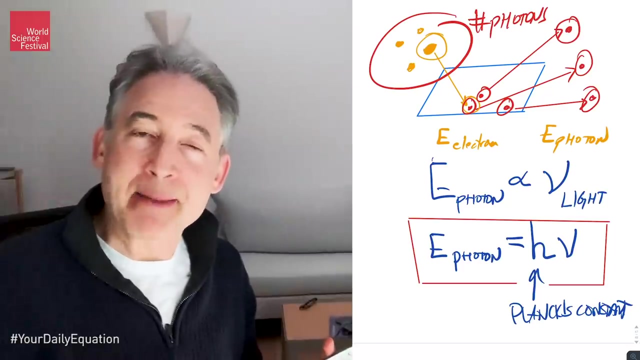 of the light. Well now, that's quite obvious. The intensity of the light is nothing but the number of photons. Higher intensity, greater number of photons, Greater number of photons, Greater number of collisions with electrons. Greater number of collisions, Greater number of electrons that will be emitted. 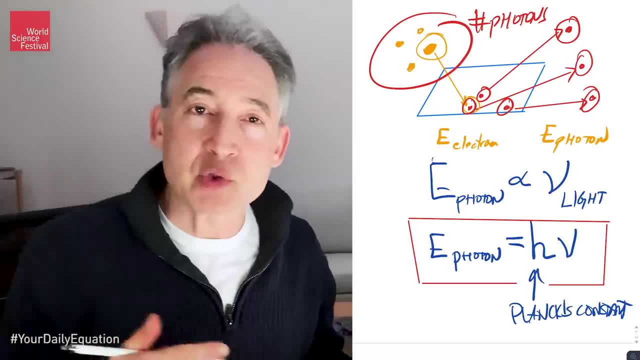 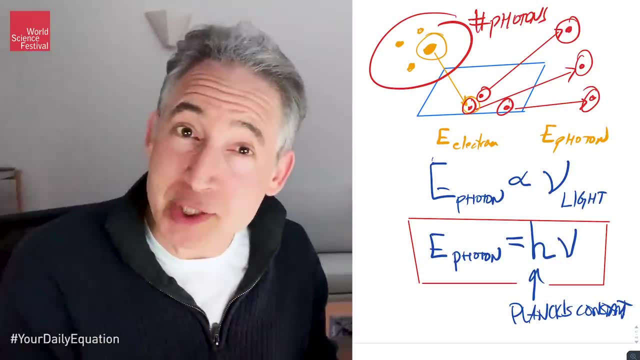 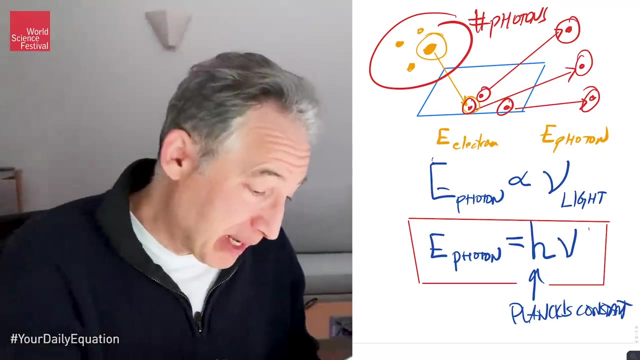 So that's why the number of ejected electrons is determined by the intensity of the light, because the intensity is just the number of photons and the kinetic energy of each of those electrons. at least the maximum kinetic energy that any of them can have is determined. 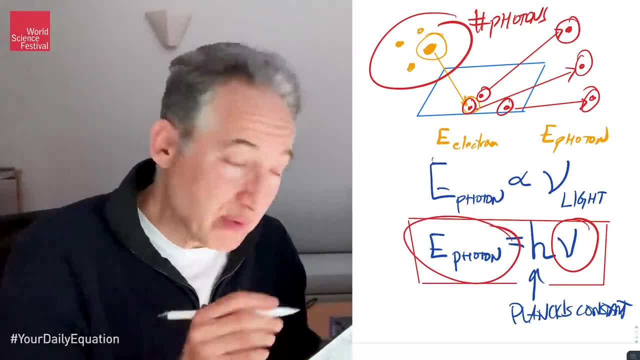 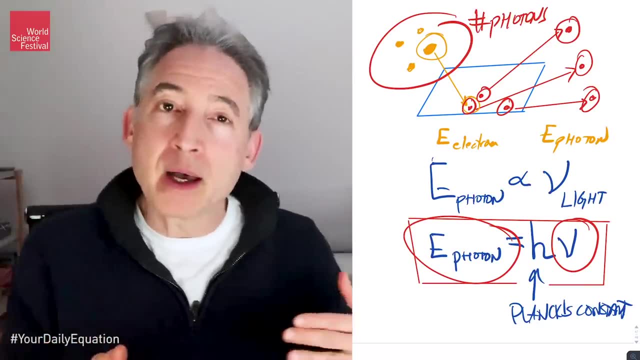 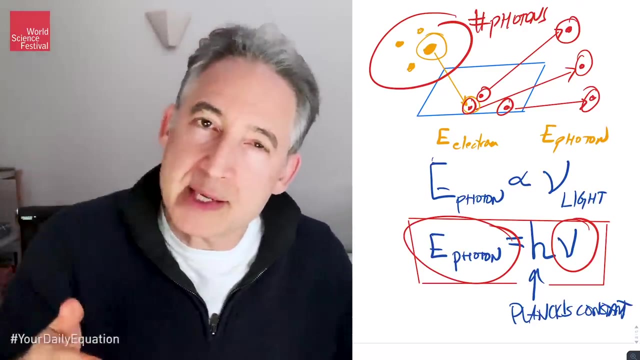 by the color of the light, Because the energy of each photon is proportional to the frequency of the light. So it's kind of a beautiful blending of wave-like ideas. I mean, frequency, after all, is a notion that has to do with a wave. and Einstein says: take that wave-like idea and blend it into. 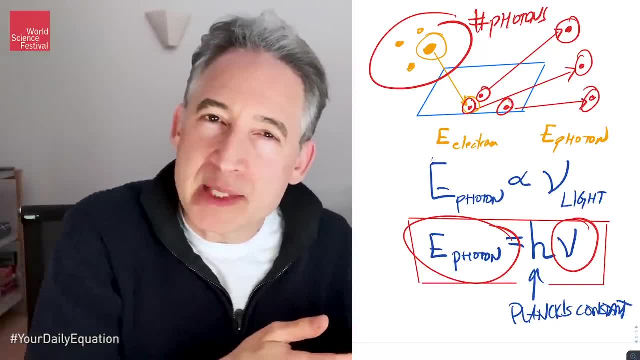 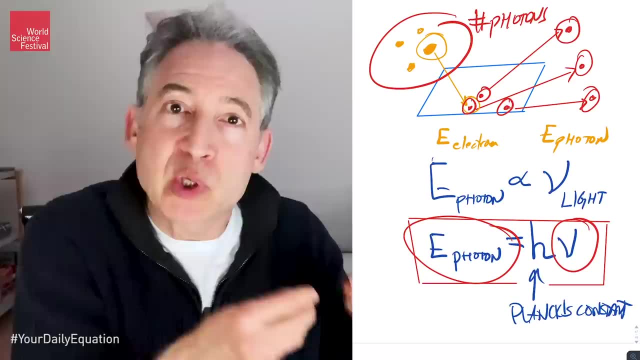 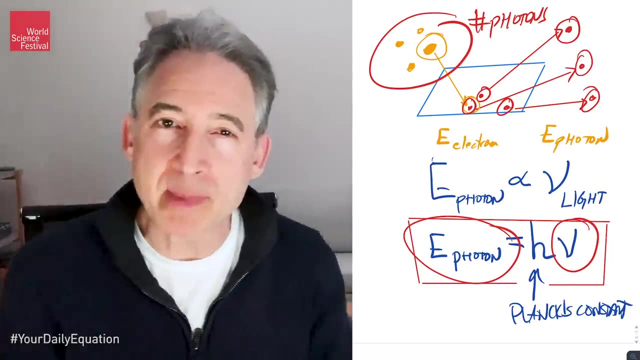 a particle description of light. So it's not quite going back to the Newtonian picture of particles of light. It's not quite using the pure wave-like description of light that came to us from James Clark, Maxwell and previous analyses and experiments. Einstein kind of blends them together using a wave-like concept. the frequency of the 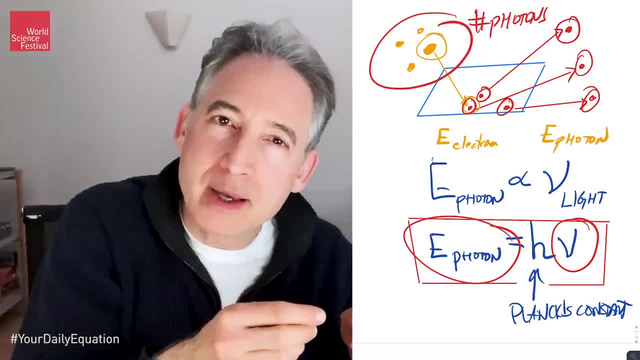 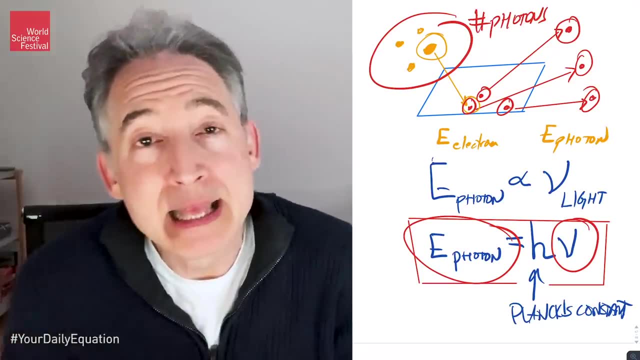